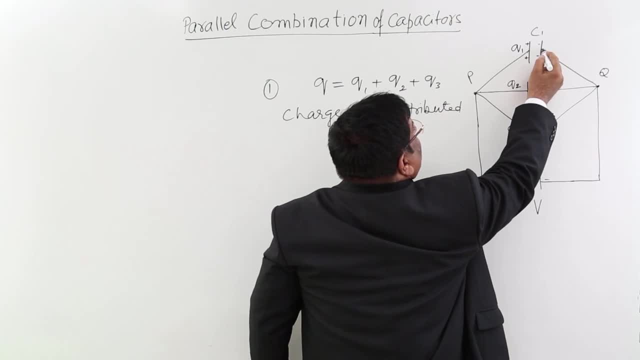 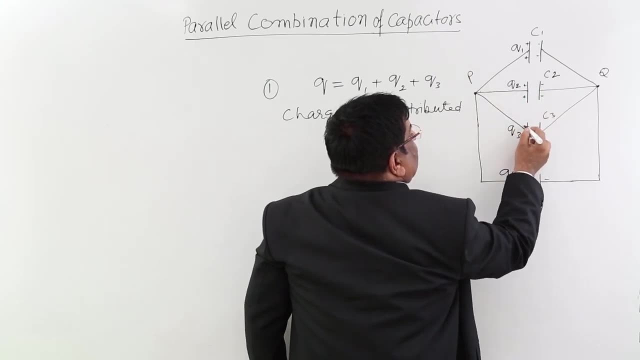 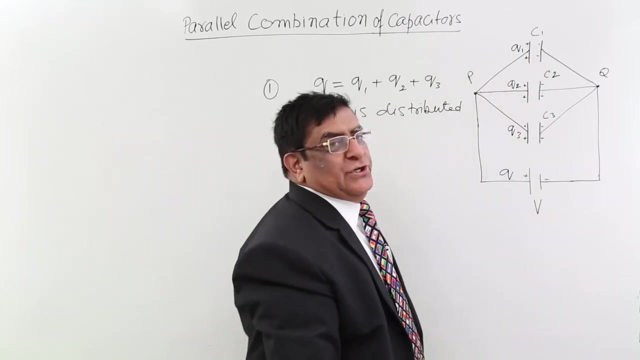 will be minus charges here and its plus will be repaired and they will go to this minor. So, everywhere what we find, this capacitor is charged. A potential develops across it. How much is that potential? Now, this is a thing you must understand. This battery, this 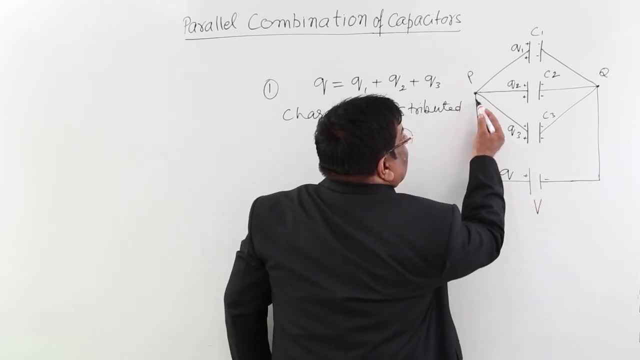 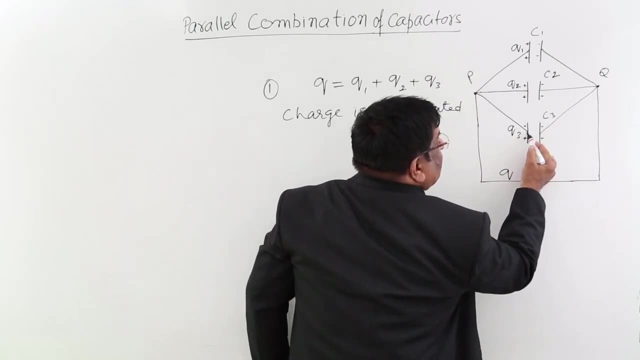 has potential difference V. This one plate is connected with conductor to this plate. This is connected with this plate. So these two plates are directly connected to these two plates. So potential has to be V because this is V. this is V connected with this. 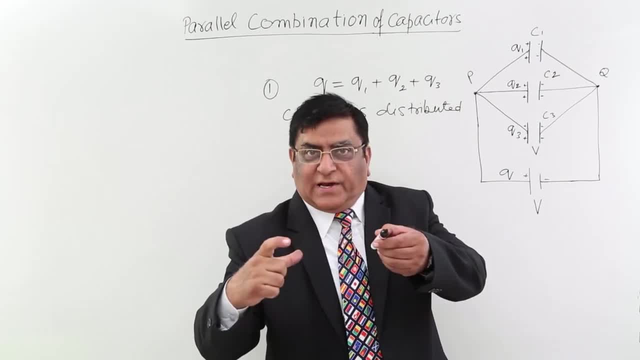 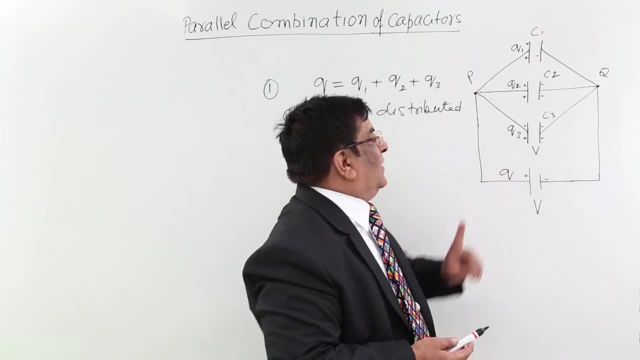 If you have a battery of potential difference V, you take these two wires, what will be the difference of potential between the two V? that V is there, So it has got potential difference V, but the same logic we apply here. This one. 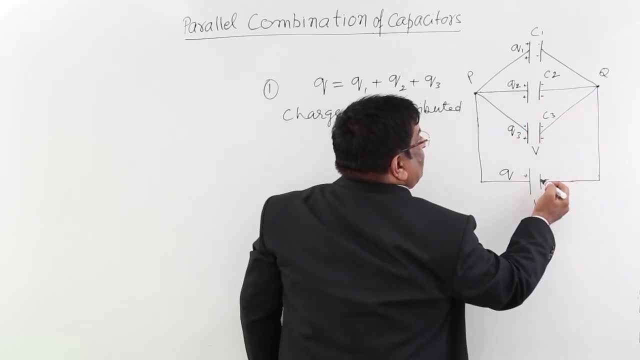 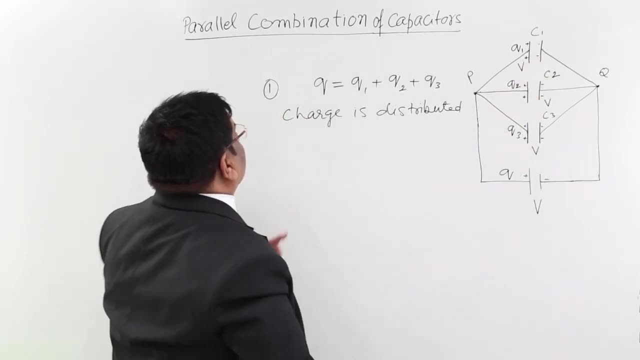 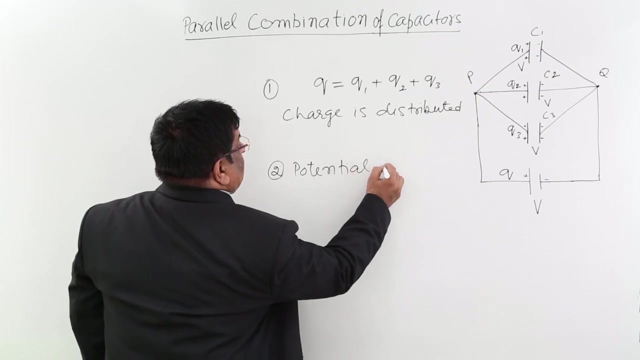 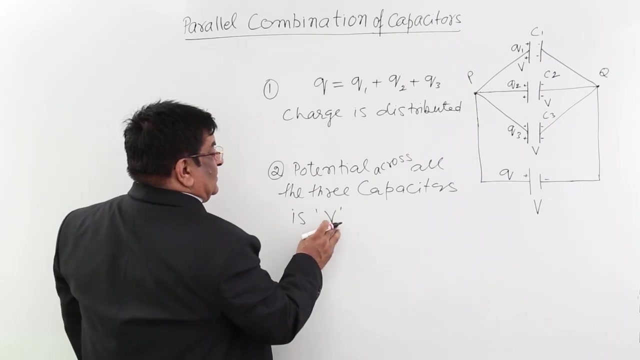 is connected directly with plus, this is connected directly with minus. So here potential difference is V and for this also potential difference is V. So in this case, potential on all the 3 plates, all the 3 capacitors, potential across all the 3 capacitors is V. 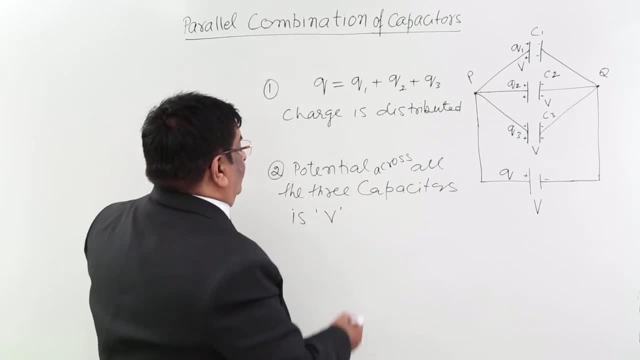 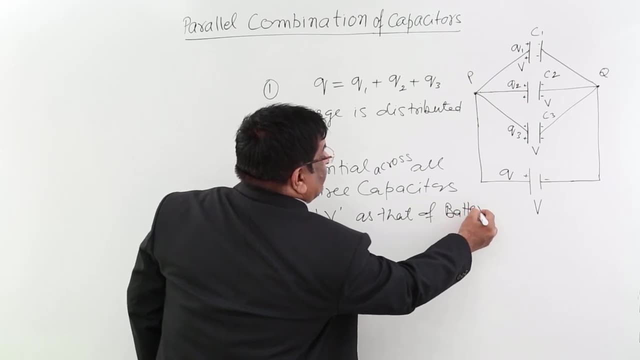 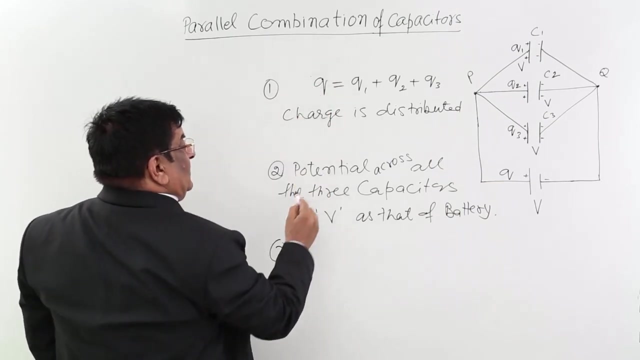 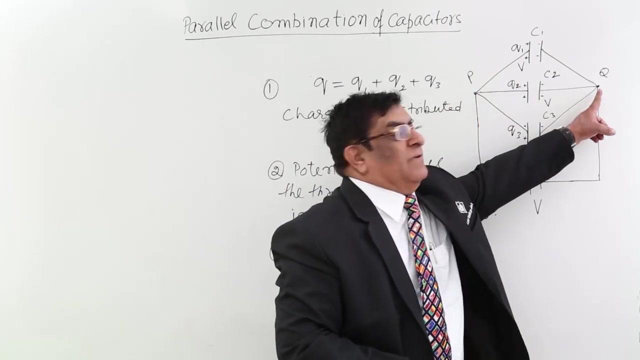 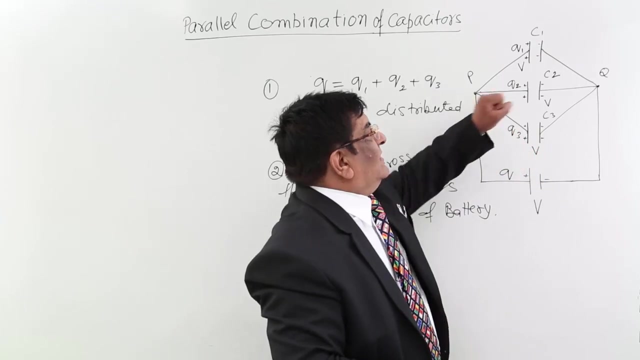 potential across all three is V. So thanks V. same as that of battery. we have discussed charge. we have discussed potential. now we will discuss capacitance. what is the equivalent capacitance between P and Q? what is capacitance? the charge divided by potential is the capacitance how much it will need. okay. 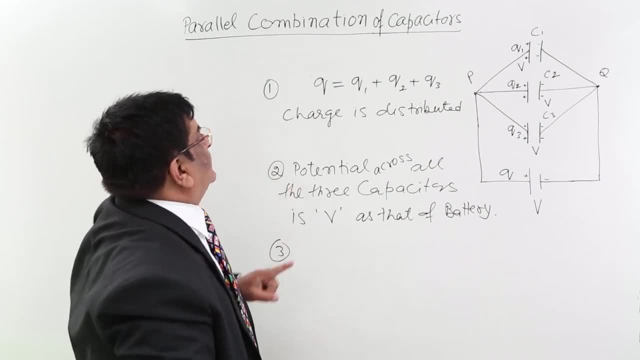 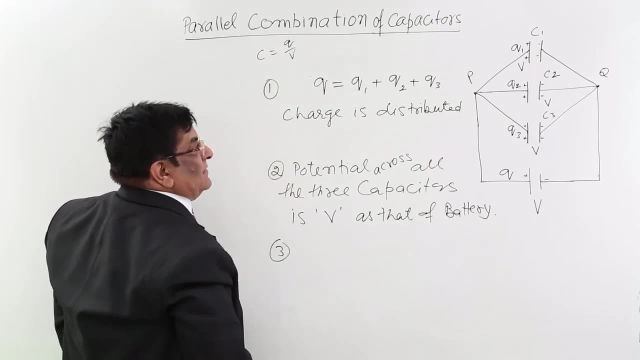 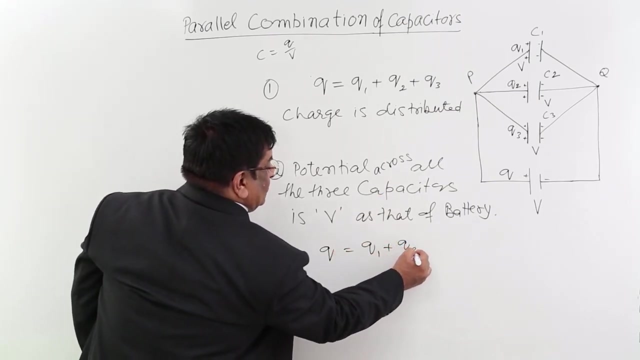 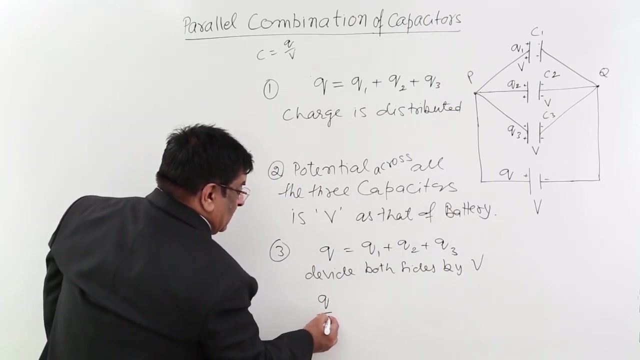 So how we will find out capacitance? we know the fundamental formula: that C is equal to Q upon V. in first case we have given charge Q, which is Q1 plus Q2 plus Q3. divide both sides By V. if we divide both sides by V, this will be: Q upon V is equal to Q1 upon V plus Q2 upon. 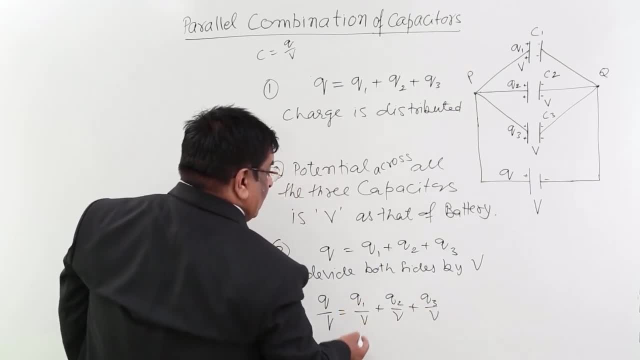 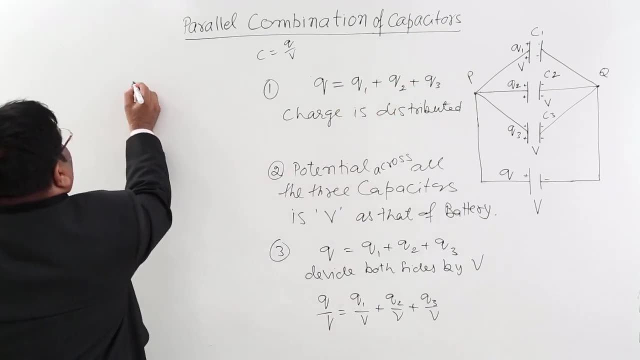 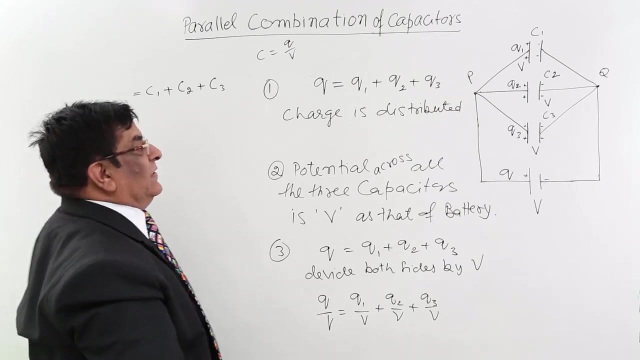 V plus Q3 upon V, now Q1 upon V, Q upon V is C, so Q1 upon V is C1. so this is C1 plus this is C2 plus this is C3. and what is this Q upon V? where is the V applied? V is applied between: 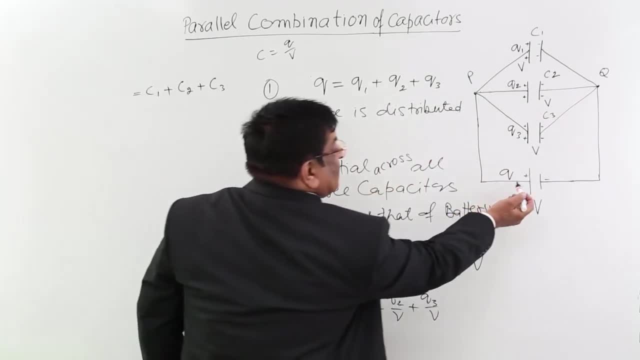 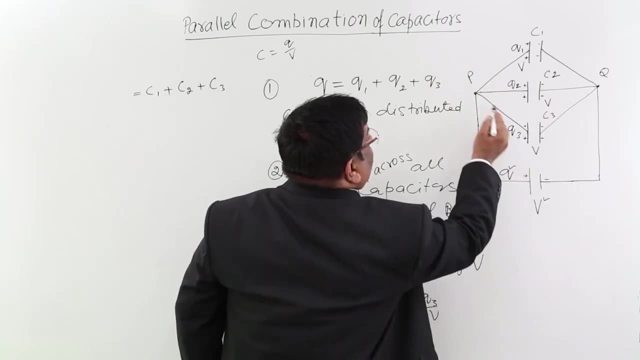 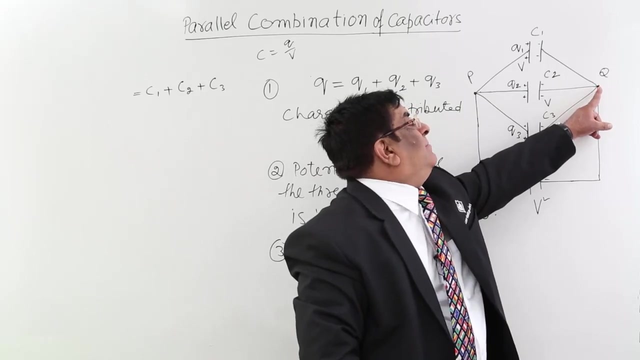 P and Q. so Q is the total charge given. so total charge between P and Q is Q, total potential difference is V. so capacitance between P to Q. if we take capacitance between P to Q, what does that mean? capacitance of the total system. this we will call equivalent capacitance of. 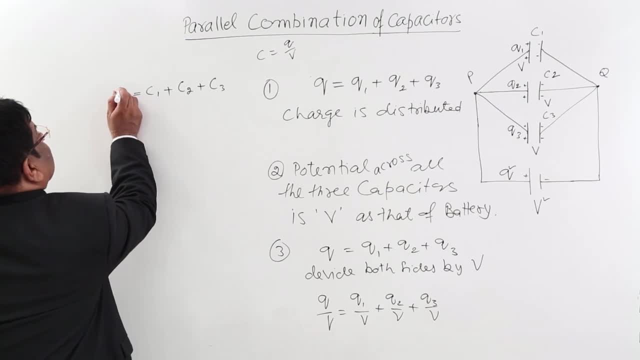 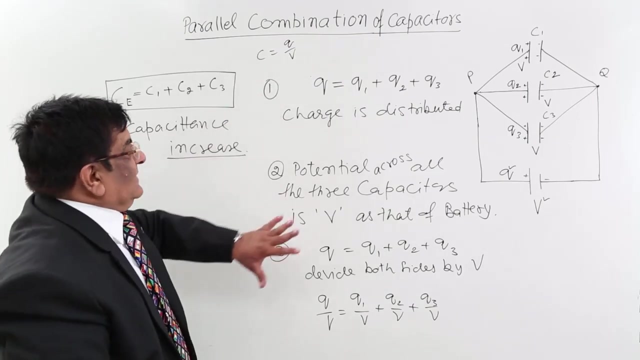 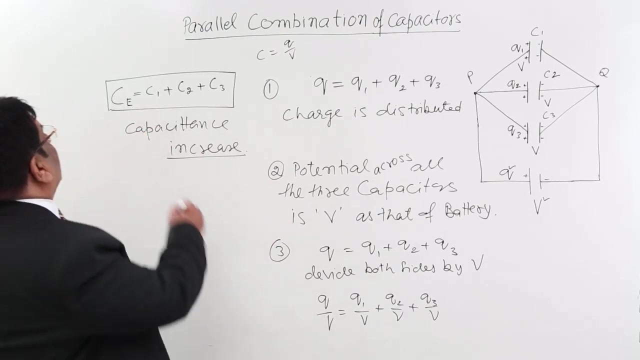 the system. so this is equivalent capacitance of the system, C equivalent. so this is our formula for C and this is a very simple addition. that means all the capacitance will be added up to give an equivalent capacitance. So capacitance increase. So this is charge condition, this is potential condition, this is capacitance condition. and 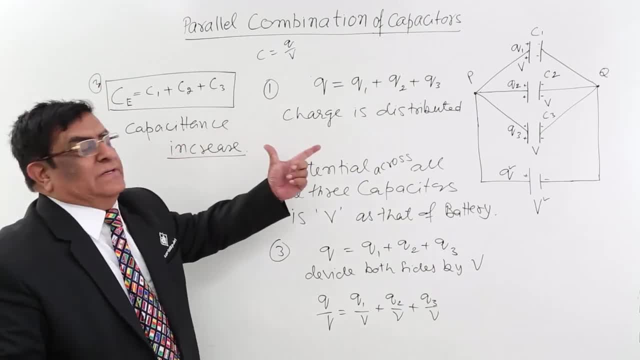 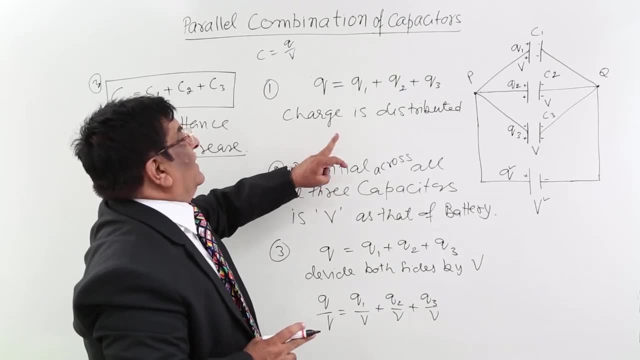 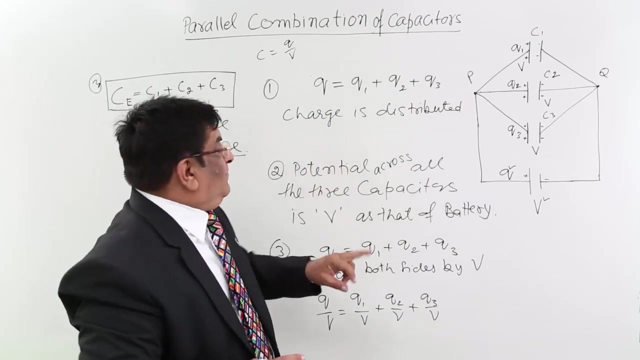 you must remember these 3 conditions, as you remember in the series. okay, let us see the series and compare the two. In this charge is distributed In series. charge was same in all the 3 here. potential is same in all the 3 in that potential. 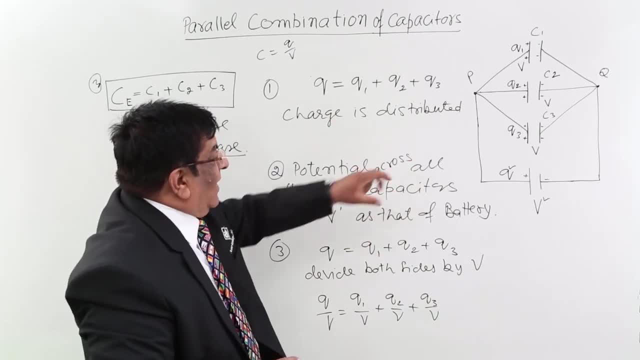 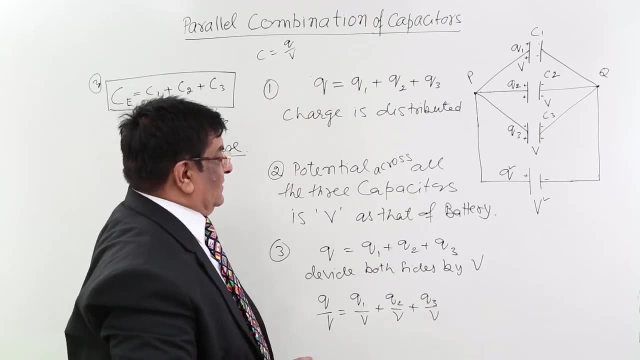 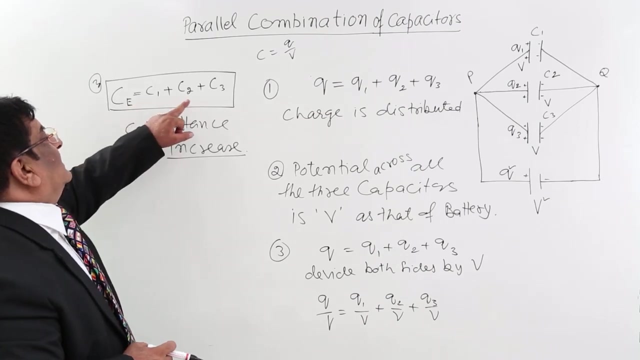 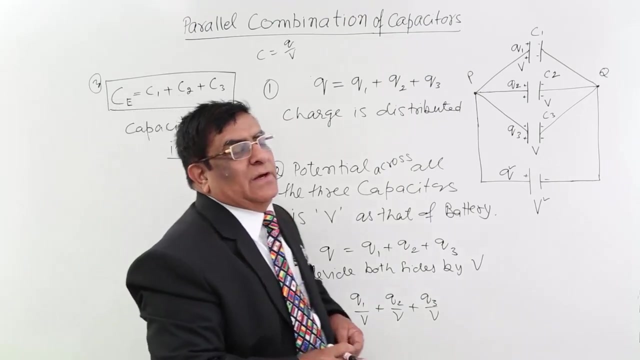 was distributed. so here, in parallel potential is same charge distributed in series charge, was same potential distributed. okay, capacitance in series, capacitance decrease. in parallel capacitance increase. this is the formula in this. So this is parallel capacitors. Now here, how do we calculate the things which are unknown? 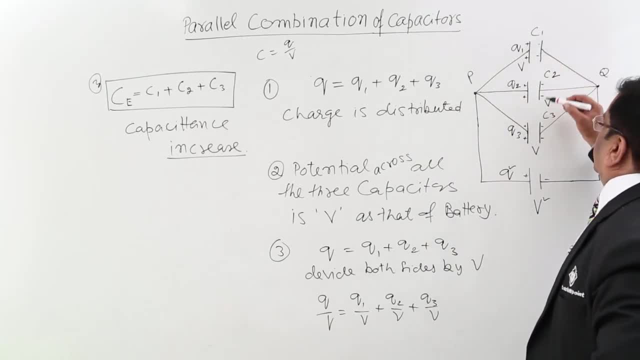 What is unknown. We have 3 capacitors- C1, C2, C3- and a battery of charge. V is applied to it. That means C1, C2, C3 and V. these are the 4 quantities which are given to us. 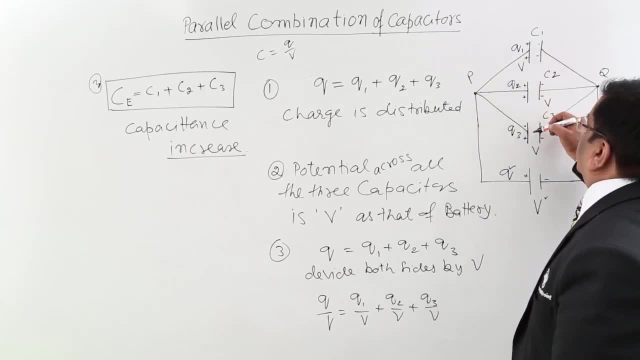 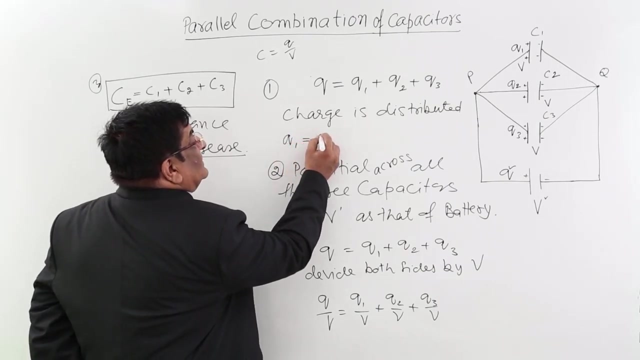 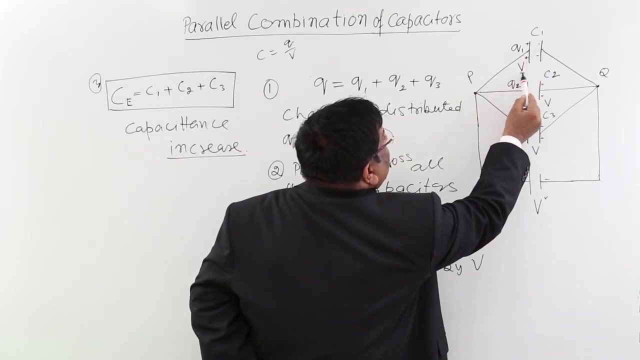 What we are asked. Find out charge on each capacitor. So that is very easy. Charge on first capacitor, Q1 is equal to Q1.. How will you find out? Answer: C1 is given, V is given. This is capacitance C1 and its potential is V. and what is the relation between V, C1 and Q1? Q1 is equal to C1 V. Q2 is equal to C1 V. Q2 is equal to C1 V. Q3 is equal to C1 V. Q4 is equal to C1 V. Q5 is equal to C1 V Q6 is. 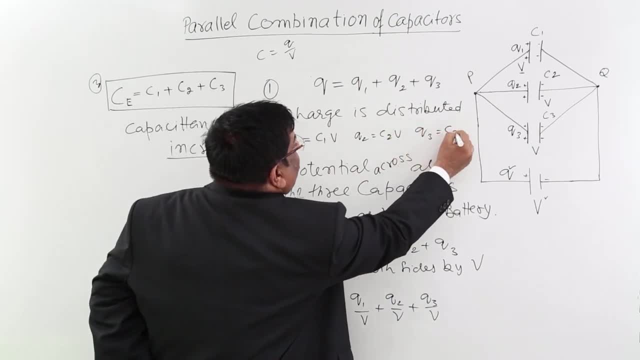 equal to C1 V, Q6 is equal to C1 V, Q7 is equal to C1 V, Q8 is equal to C1 V, Q9 is equal to C1 V, Q10 is equal to C2 V And Q3 is equal to C3 V. You have calculated all 3.. Now, if it is asked, 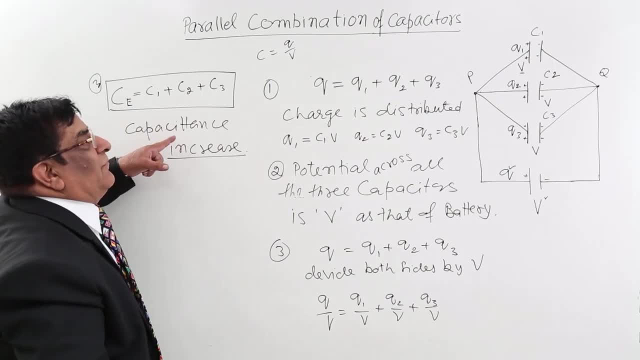 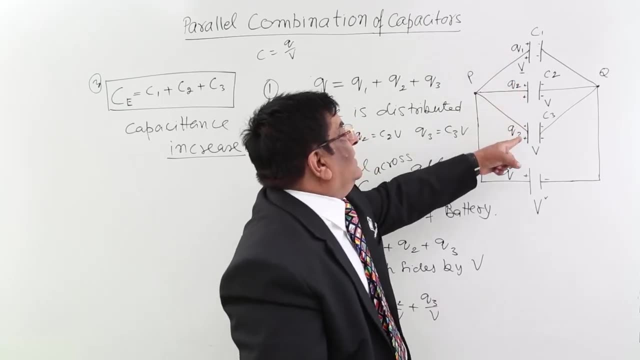 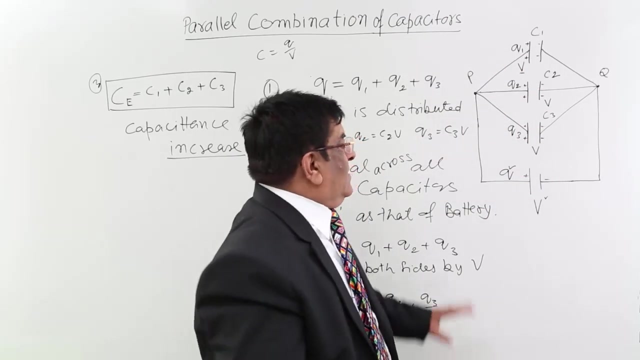 what is the total capacitance? Use this formula, you will find total capacitance. Then you are asked: how much is the total charge drawn? Add up all the 3, you will get the total charge drawn. How much is the potential? V, V, V is the potential. So this is our combination. 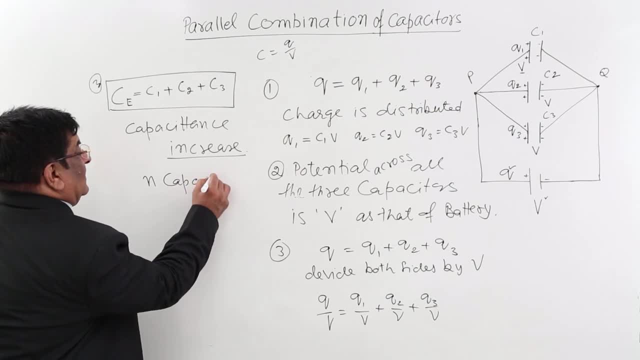 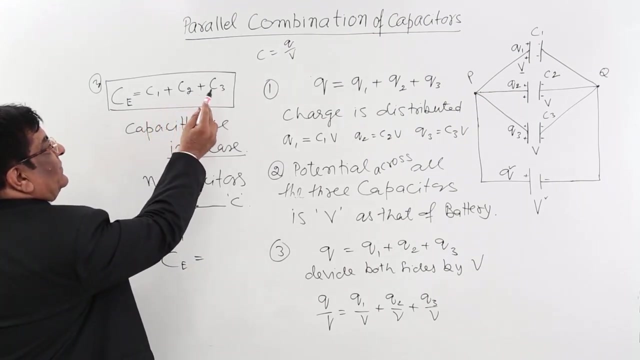 So this is our combination, And now, after you see that V is equal to C1 V- V, you will be able to calculate the total charge drawn using the formula showing here. And so V is equal to C1 V, V. V2 is equal to C1 V- V1.. Q1 is equal to C2 V- V2 is equal. 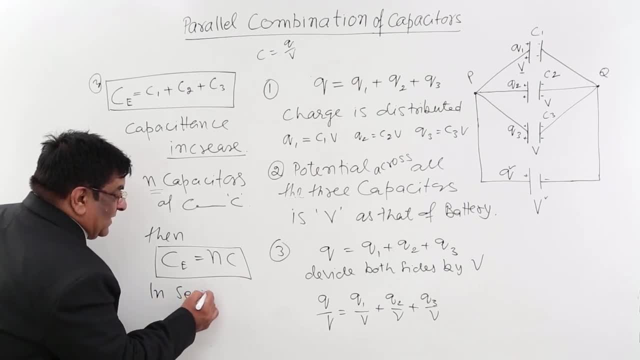 to C2 V, X, C1 V And you have calculated the total charge drawn. You can see that the total, If there are n capacitors, then 1 upon C equivalent is equal to 1 upon C1,, 1 upon C2,, 1 upon C3. 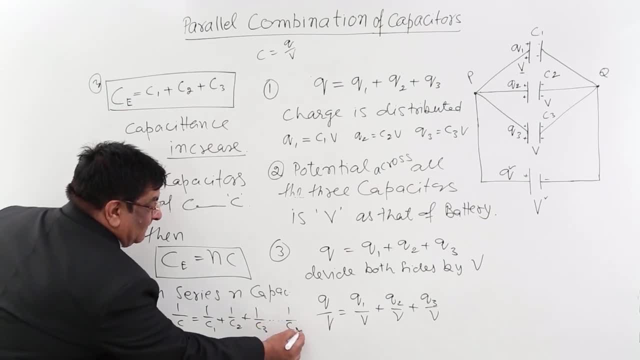 and this will keep on. 1 upon Cn. What will be the total of this? Okay, if all are C, if all are C, then this will be C, C, C and C. How many Up to n? so this will be equal to n upon C. 1 upon C equivalent is equal to n upon C. okay. 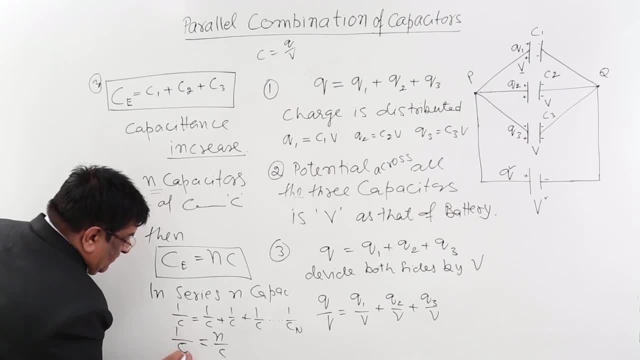 Okay, so C equivalent is equal to C upon n. This is a very important formula for our calculation purpose. This is in series. If there are n capacitors, each having capacity C, what is the total equivalent? Answer: C divided by n. 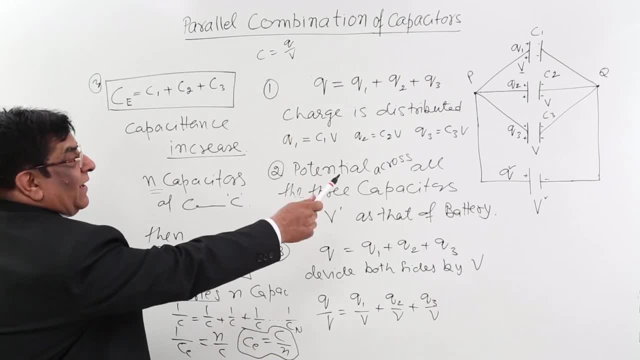 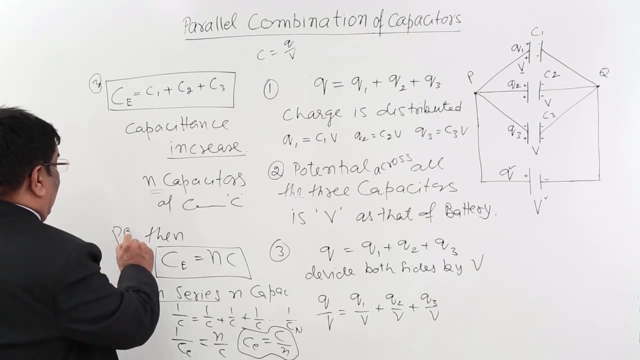 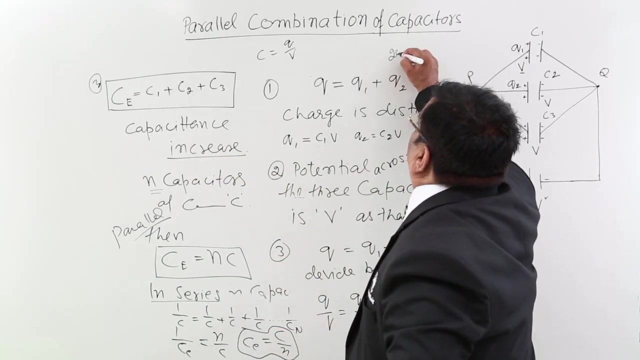 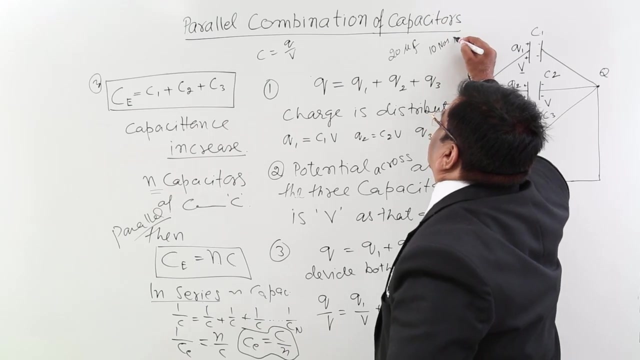 If there are n capacitors fitted in parallel, what is the equivalent Equivalent capacitance? n multiplied by C, So in parallel, multiplied by n in series divided by n. okay, Like I ask you, there are capacitors of 20 microfarad and we combine 10, 10 numbers in series, in series. 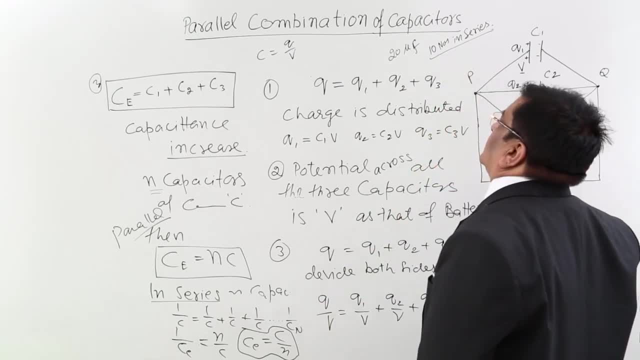 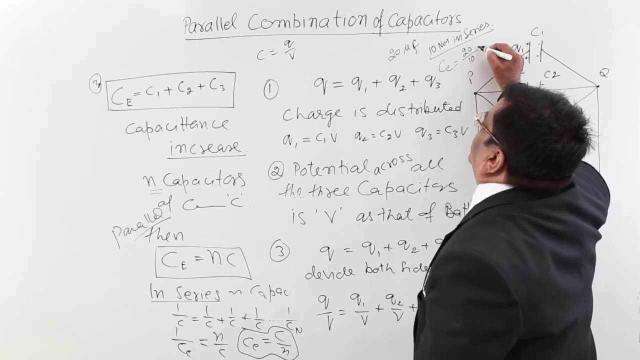 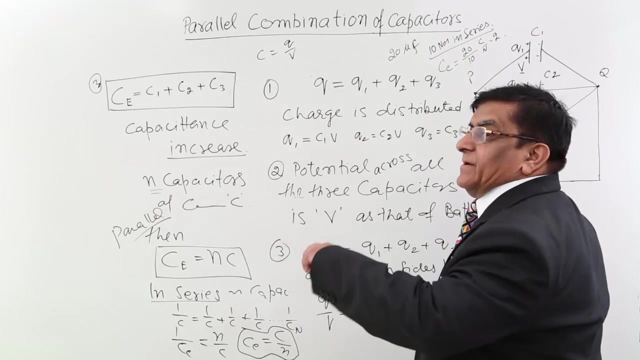 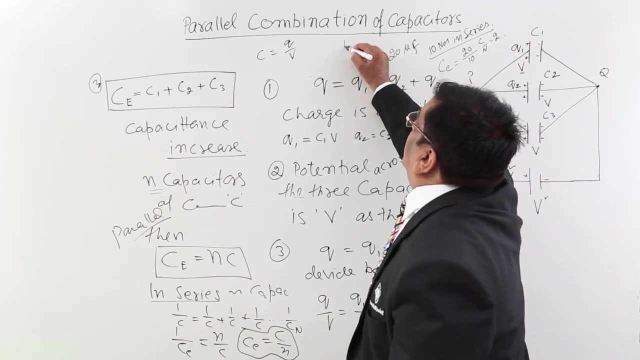 What is the equivalent capacitance? So answer: 20 divided by 10.. This is C equivalent, What we have used, C upon n, So this is equal to 2.. Other, if there are 10 numbers capacitance joined in parallel, parallel, and each is 20 microfarad.